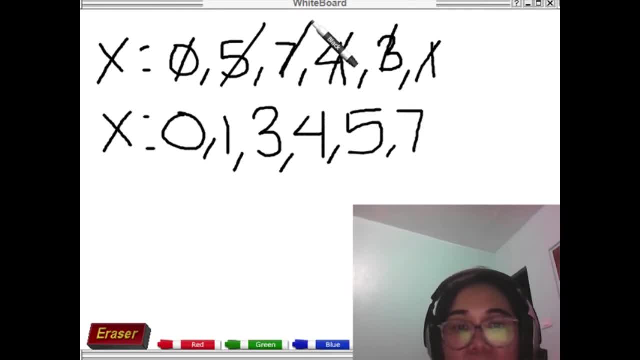 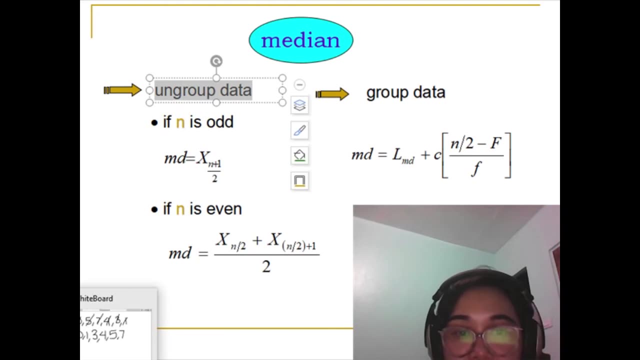 Okay, then we have the last observation, which is 7.. So take note that the data now is arranged from lowest to highest. You will now recall our formula for n-group data. Okay, so we have to consider the number of the number of observations that we have in our example. 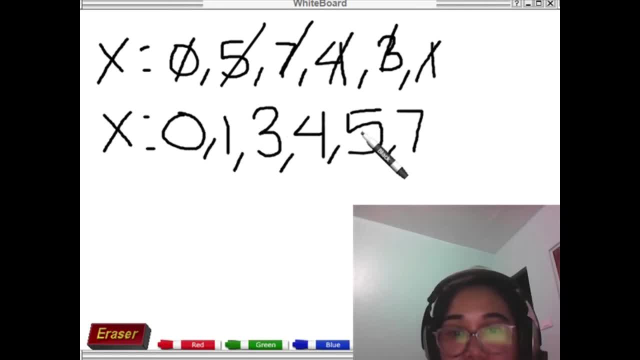 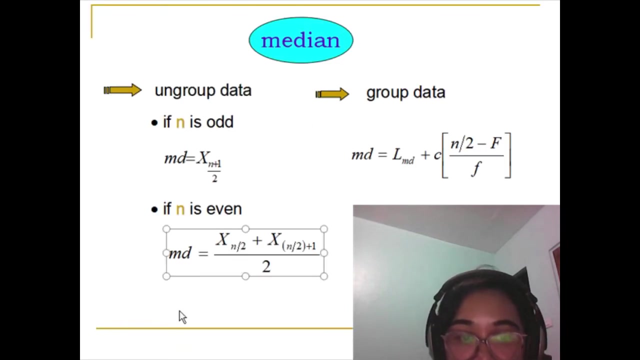 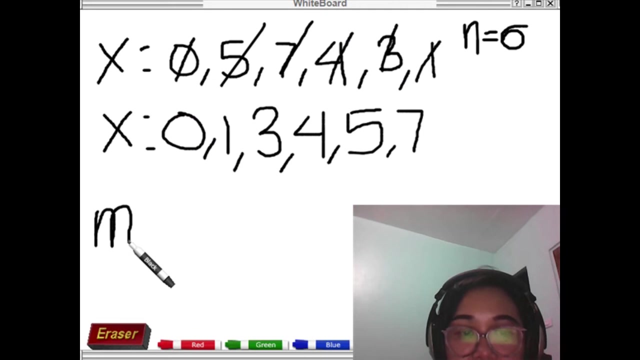 so we have one, two, three, four, five, six. our n is six. let's have it here here. okay, take note that six is an even number. okay, so we have to use this formula. okay, so our median is equal to x sub n over two. okay, so let us replace n here with six, because our n is six, okay, plus. 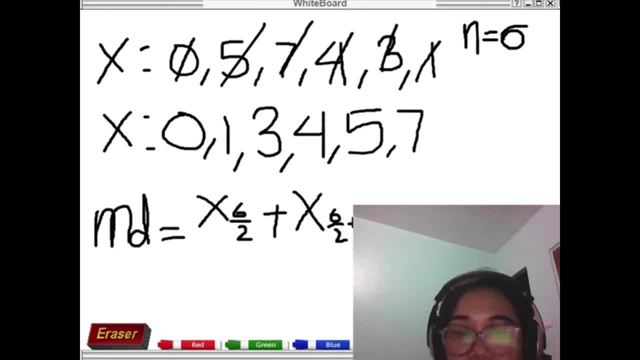 plus one, okay, then all over two, okay. so we have x sub six over two. six over two is three, so x sub three plus we have sixty five by two plus one, that is x sub four divide by two. okay, so maybe we could use this space here. 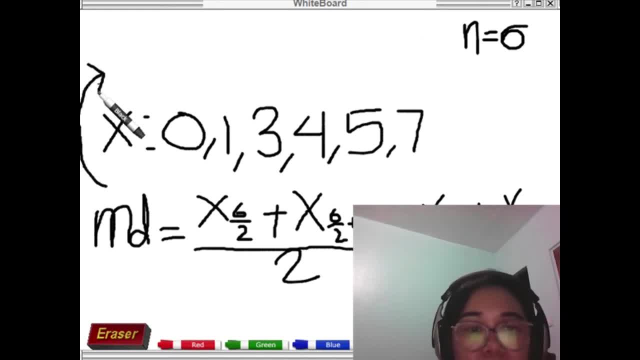 okay, let's have this arrow. okay, so median is equal to this: x of three is the third observation and this x of four is the fourth observation. okay, so let's locate what is the third observation. we have one, two, three. so we have three, so we have it here: three. then the fourth observation is one, two, three, four is four. 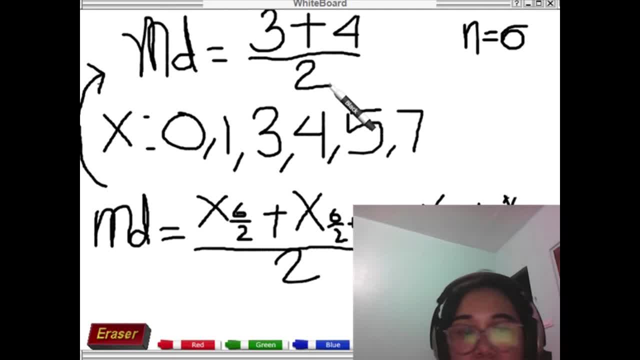 okay, so we divide it with two. let us erase this. we already know that n is six. okay, so what do we have? three plus four, divided by two, is equal to seven. divide by two, which is equal to three point five. wait, okay, let's have point here. 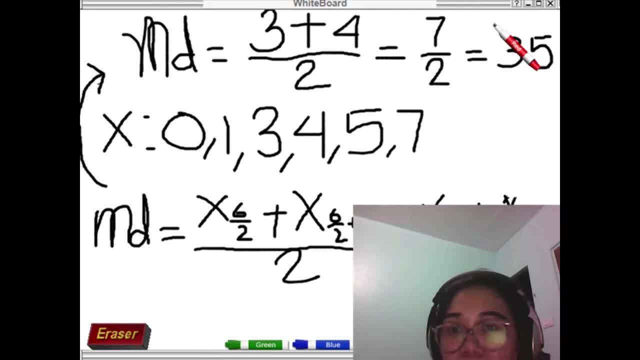 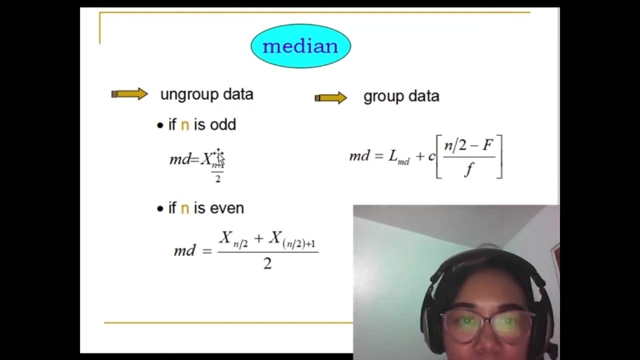 then we have five. okay, so the median value is 3.5. okay, how do we interpret 3.5? so we say that 50 percent of this given data set is below 3.5, or 50% of this given data set is above 3.5? say, for example, our n is at here. 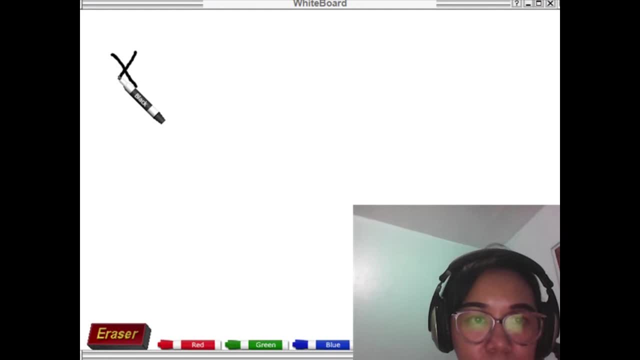 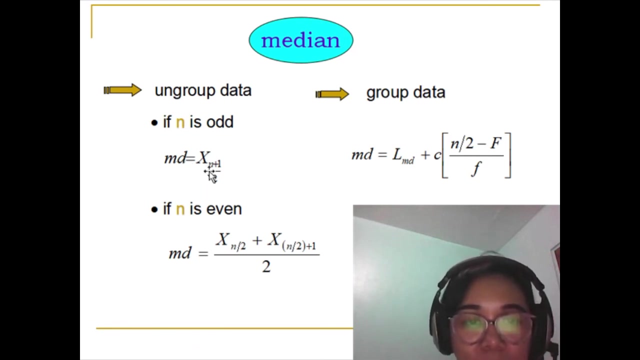 okay, so we have 1, 2, 3, 4, 5. our n is 5, so 5 is an odd number. let us recall the formula of the median value when n is at. so that is simply x sub n plus 1 over 2. you go back here. 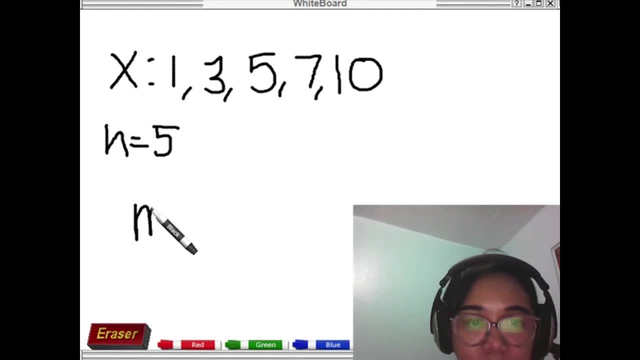